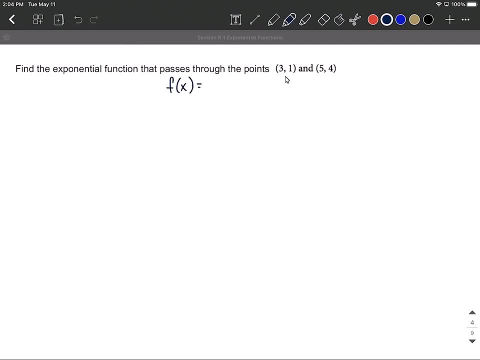 steps as we go through. First of all, we know it's an exponential function, so that means it has to fit into this format: a times b to the x power. So what I'm going to do is first create two equations here based on these ordered pairs that we're given. Right, we have three as an x value goes with. 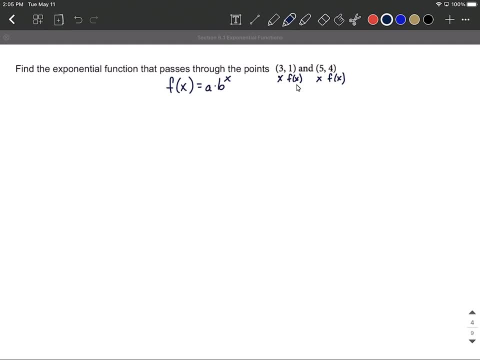 one for an f of x or y value. So one equation we can get is: plug in one for f of x, plug in three for our x. A second equation can be used in the ordered pair: five, four. So that's going to be: plug in four for f of x equals a times b to the fifth power. plugging in five for x in our general 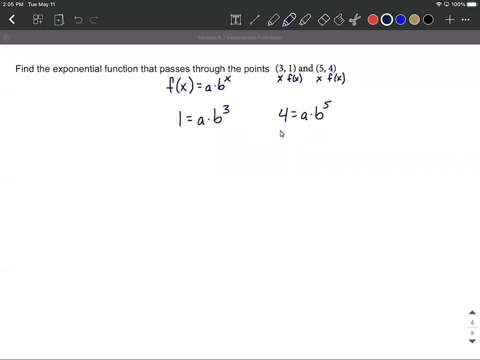 exponential function. All right, now we have two equations and two unknowns. Sometimes this is referred to as a system of equations, So I want to introduce four steps that can get us through these systems of equations. This method is referred to as the substitution method. 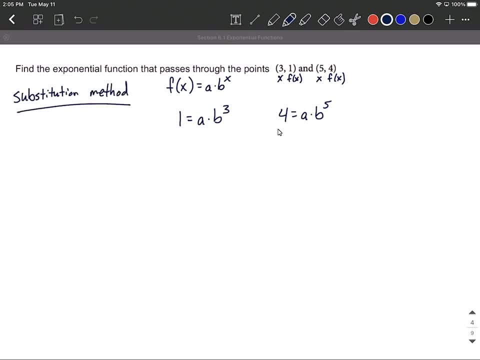 And I'm going to write the steps off to the side as we go through them. So the very first step is: we have two equations, two variables. We want to solve one equation for a variable. Okay so, two equations, two variables. I like to pick out whichever equation I think is going to. 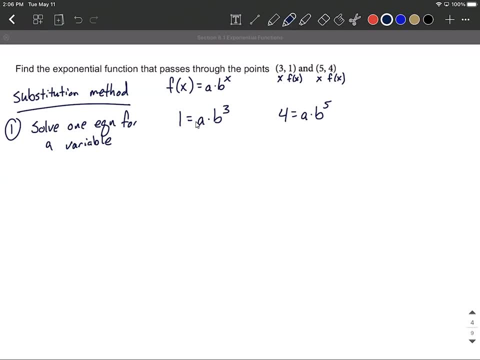 be easiest to solve for a variable. I think solving for a in either one of these is probably going to be easier to solve for than for b. I'm just going to stick with the left equation as I wrote it, because it's got a little bit smaller numbers. So to get a on one side by itself here. 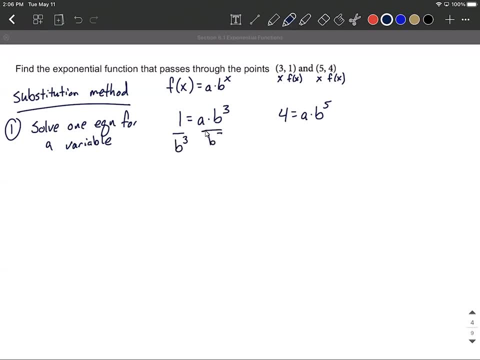 we'll just divide both sides by a And then we're going to do the same thing for the other side, So that'll put a on one side by itself, over b cubed. end of step number one. Okay, step number two. we are going to substitute: 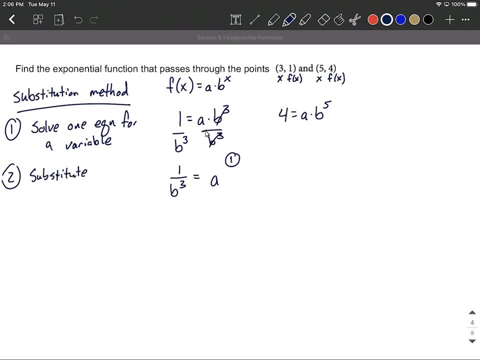 this is why it's called the substitution method into the other equation. Okay, so what I mean by that is: we know a is supposed to be the other equation. We know b is supposed to equal one over b cubed. We're going to take that over to our other equation. 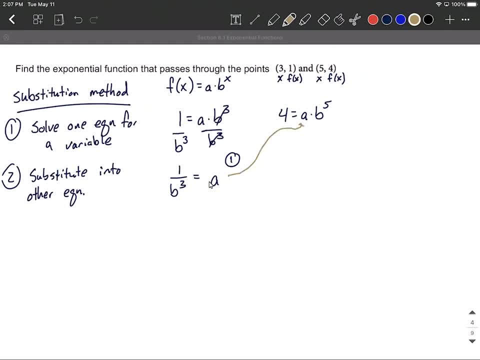 and we're going to substitute in and replace the a in the other equation with what we just said. a is supposed to equal, So at this point we can say four equals instead of a. We're going to put one over b, cubed in its spot. 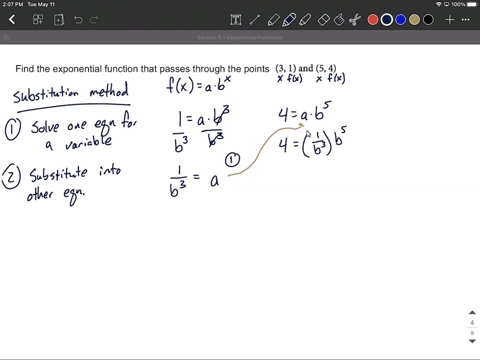 We're going to substitute in and replace this a, and that's going to be step number two. Okay, third step to this method is we've just created an equation that only has one unknown. We only don't know what b is right, so it's our only variable remaining. 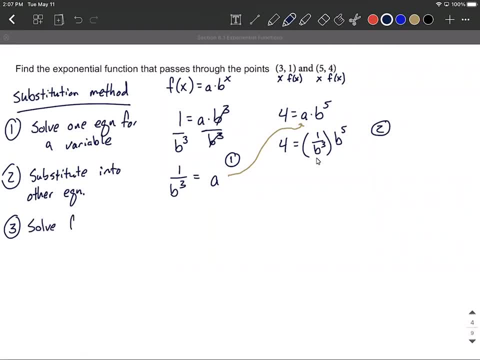 We're going to solve for the remaining variable. All right, so let's try to solve this down for b. First thing I would probably do is kind of visualize this as b to the fifth over b. So if I wanted to combine these together into a single fraction, I'd multiply einenumerators. 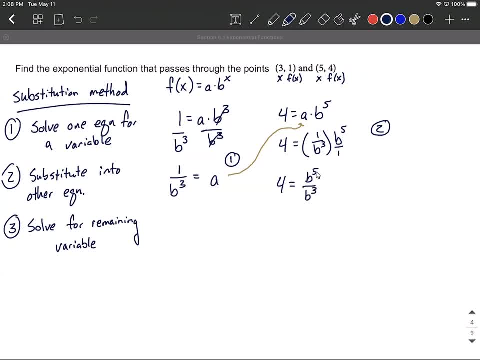 and I'd multiply denominators. Now we can simplify this down because we have b's in denominator and numerator. so I usually ask myself: where do I have more b's and how many more? Well, we have more in the numerator and there are two more, so we're going to be left with b squared in the numerator. 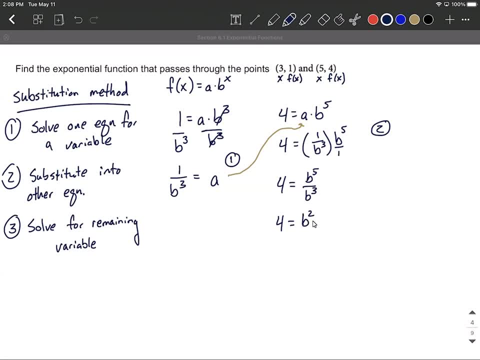 Okay, so our goal is still to solve for b. We need to get rid of the square, so let's apply a square root to both sides. it's tempting to put both the positive and negative out in front here, because that's what we're conditioned to do whenever we apply a square root to both sides of an equation. However, based 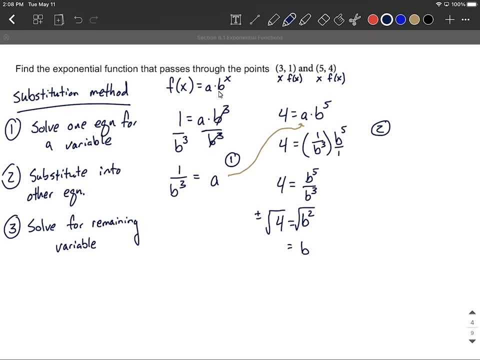 on this situation. b is the base for this exponential function and that base is not allowed to be negative. So we in this situation can actually get rid of the positive and negative case. We only need the positive case. So the square root of 4 is going to be 2.. So we know one of our variables. 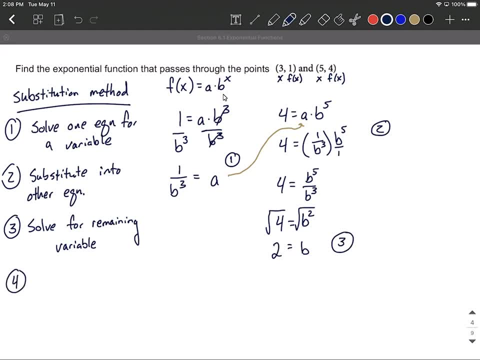 The fourth step, and probably the easiest place to go on this is we're going to substitute back into step 1.. Now, technically, you can substitute back into either one of these original equations with your b value you just found, However, in step 1, we've already done all the work to get.